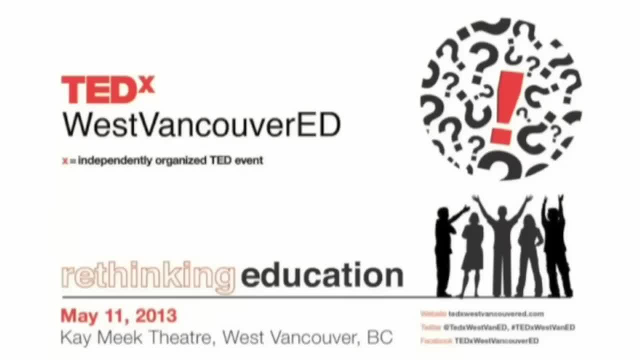 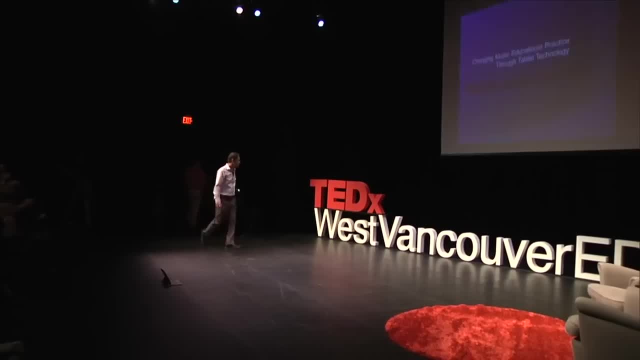 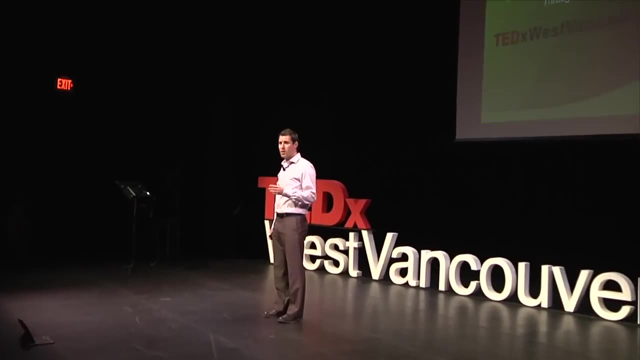 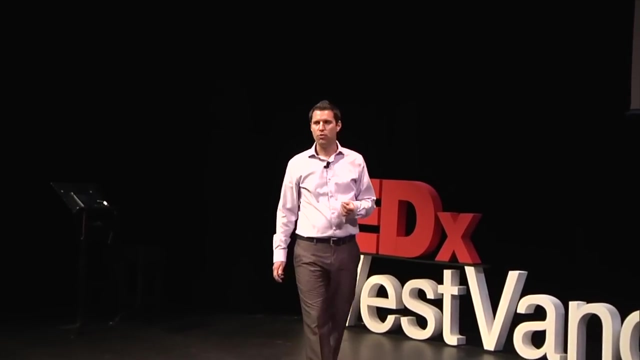 In recent years, technology has completely transformed the way that we listen to music. we share music, access it, create it and perform it. As a result, I think we should be changing the way we teach music in our classrooms, not only in what we teach, but 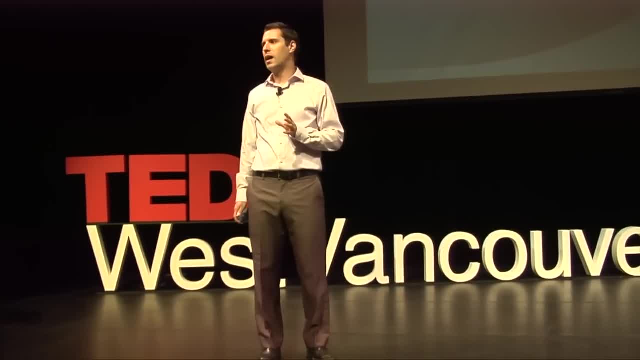 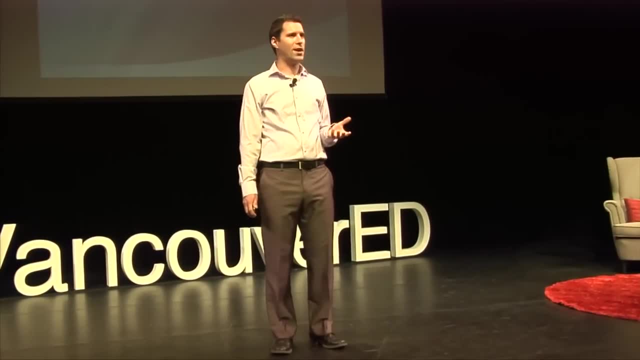 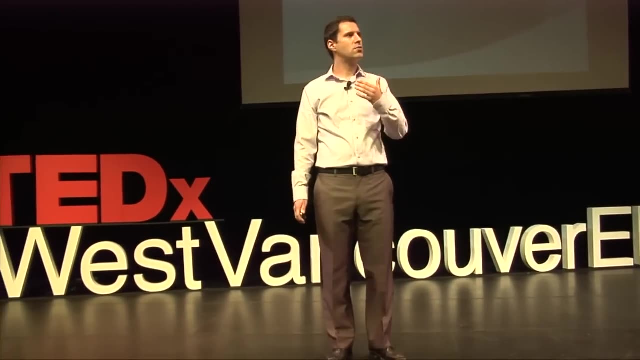 how we teach it. In the next 12 short minutes I hope to cover how I got here on my journey, which started about a year and a half ago, when I got my first new shiny iPad. I was really excited to use it and then I noticed that so were my students were really excited. 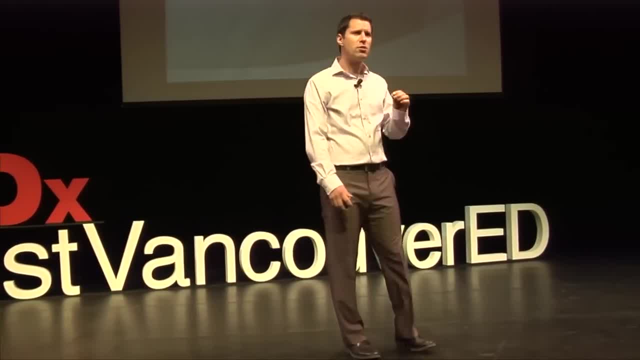 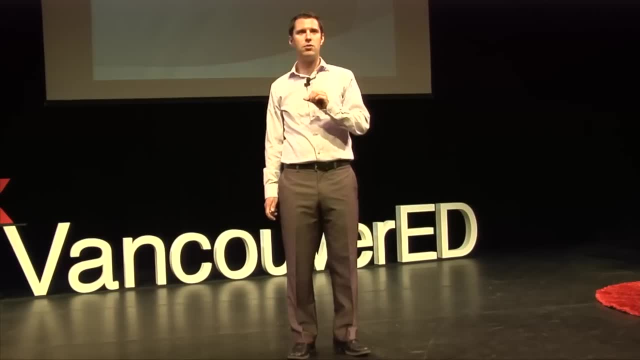 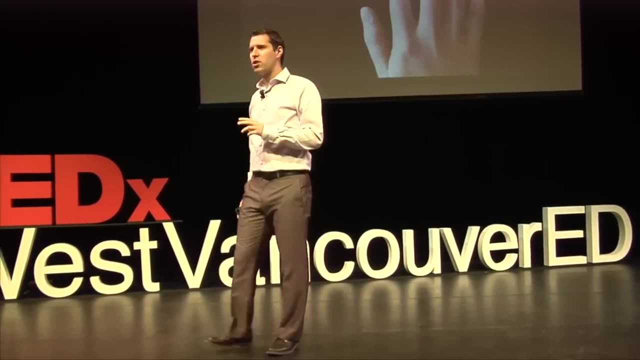 to be engaged with it And within literally about two months I had almost every single student in my school of 400. students have had a chance to either interact with the one iPad that I had or the devices that they brought in themselves. Initially, I was really 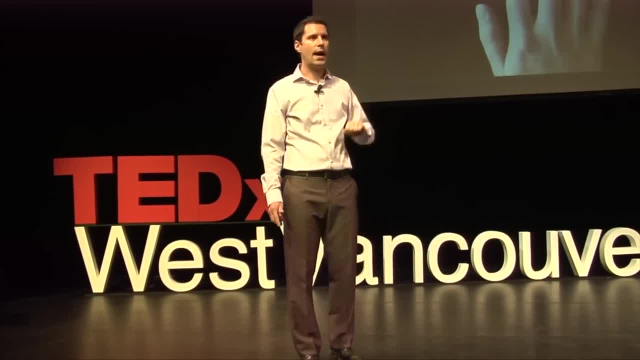 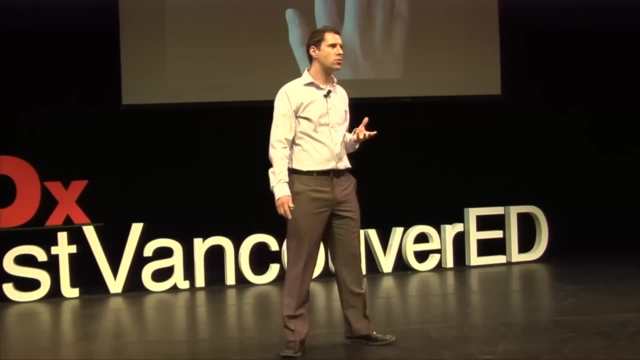 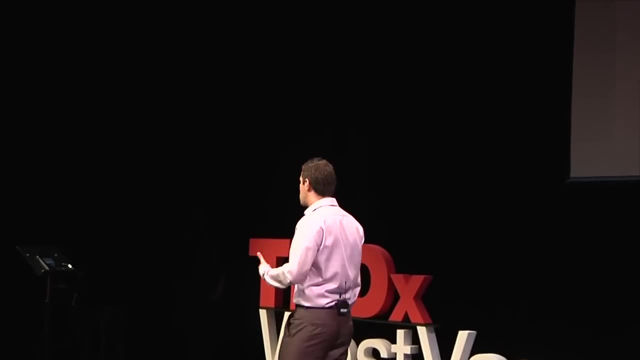 excited about the virtual instruments that you must have seen on the Apple commercials, with GarageBand, making it really accessible for all of my students- including those who had learning or physical disabilities that might have prevented them from participating fully in music class- to be able to be engaged and participate along with the rest of the 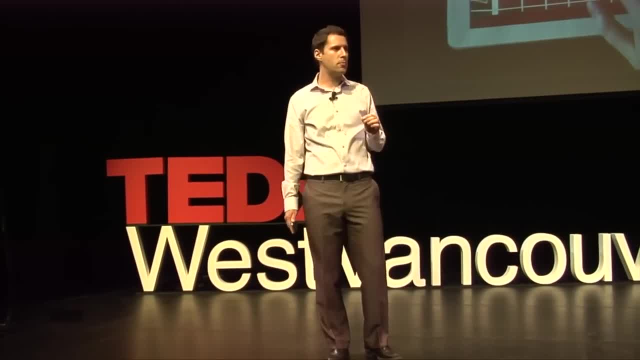 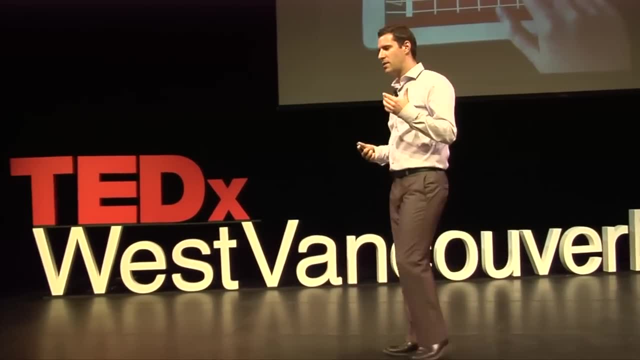 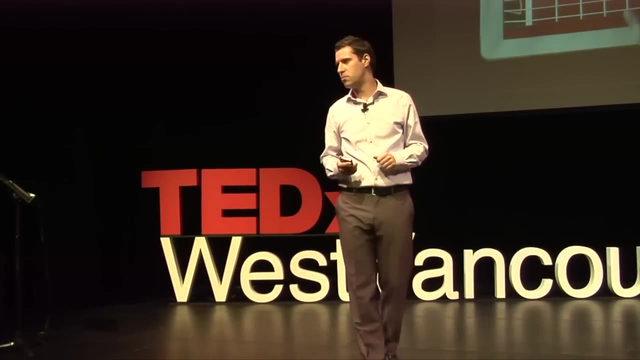 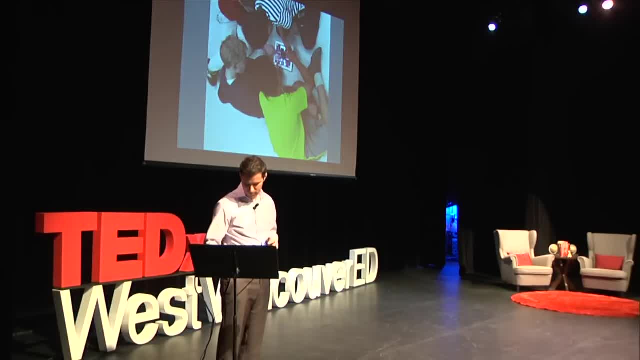 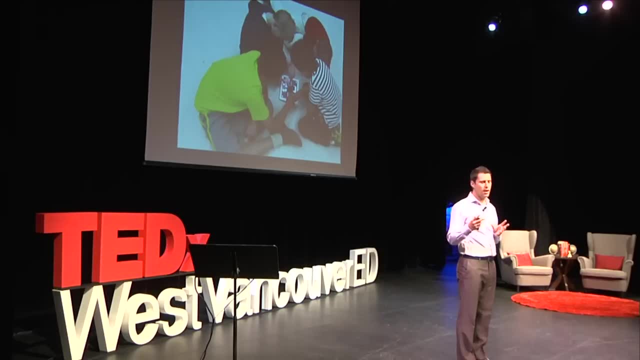 part of our lives, and it's a very important part of our lives and it's a very important Thank you. and the other thing that I wanted to talk about quickly is that the students were all singing, and not only that, not only are they singing, we're.